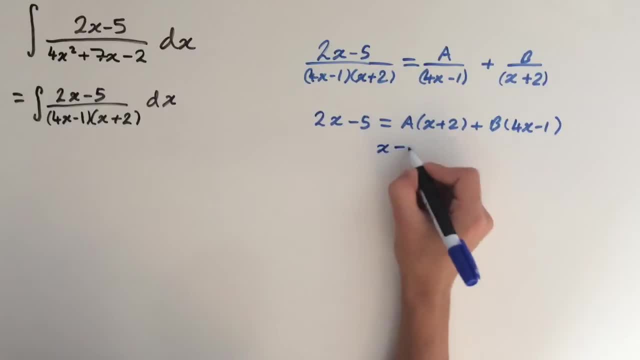 to evaluate a and b. So if we let x equal minus 2, this fraction here, this bracket here, is going to equal 0. So the value of a is going to disappear And we're just going to be left with 2 times minus 2 minus 5 equals 0 plus b times 4 times minus 2 minus 1.. So 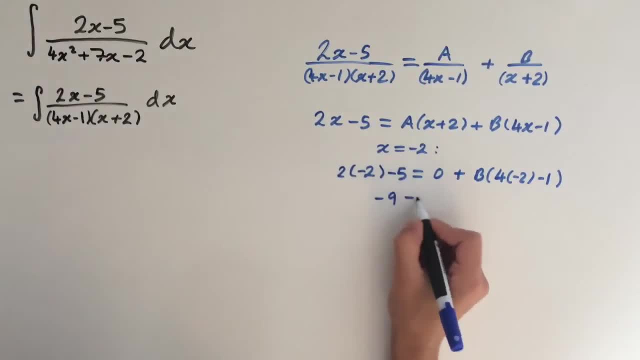 left-hand side here is going to be minus 4 minus 5, which is minus 9.. Right-hand side is going to be 4 times minus 2 is minus 8.. Minus 1 is also minus 9.. So 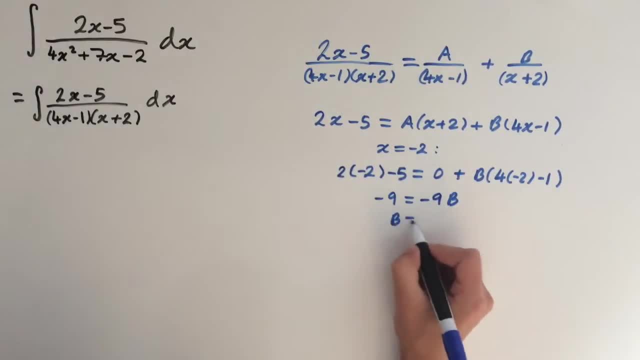 minus 9 times b. So you can see b is going to equal 1.. So now we want to let x equal a different value, So we want to make this bracket here equal 0. So x is going to have. 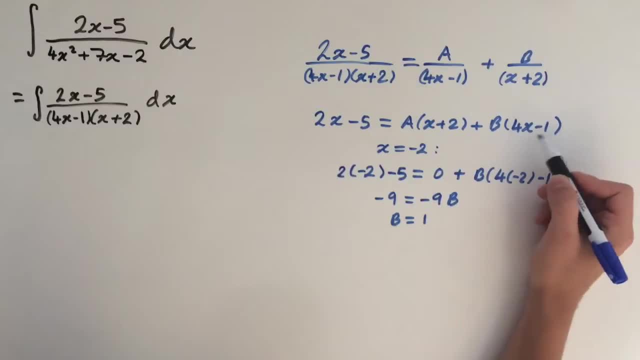 to equal 1 over 4.. So this equals 1, and 1 minus 1 is 0.. So we let x equal a quarter And now we sub it in, So 2 times 1 over 4.. So this equals 1.. And 1 minus 1 is 0. So 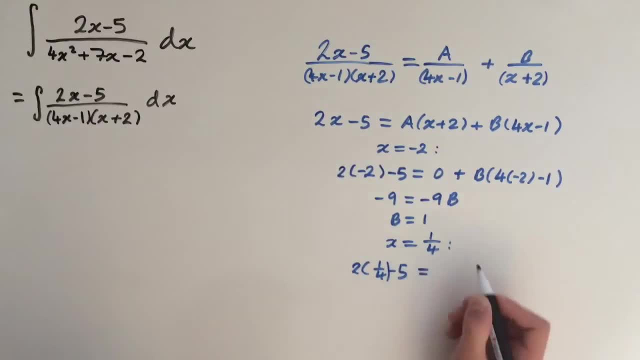 this is going to equal minus 5.. This equals a times a quarter plus 2 plus 0, because this is equal, It's going to equal 0.. So, left-hand side, this is going to be a half minus 5,. 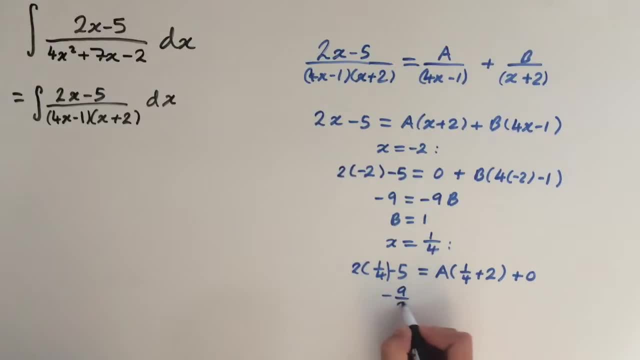 which is minus 4.5, or minus 9 over 2.. And right-hand side is going to be a quarter plus 2.. 2 we can express as 8 over 4.. So 1 over 4 plus 8 over 4 is 9 over 4.. So 9 over 4 times a, And so we need to multiply. 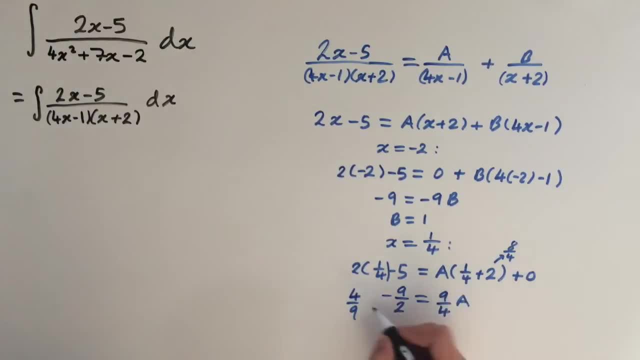 it by 4 over 9 on both sides, And these two fractions will cancel out. 9's are going to cancel out And we're going to be left with minus 4 over 2, which means a is going to be minus 2.. So now we want to sub these back into here.